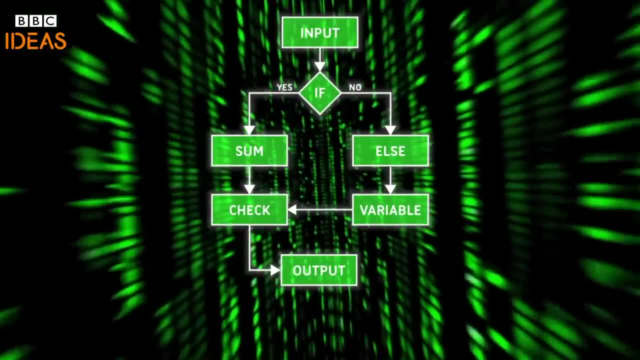 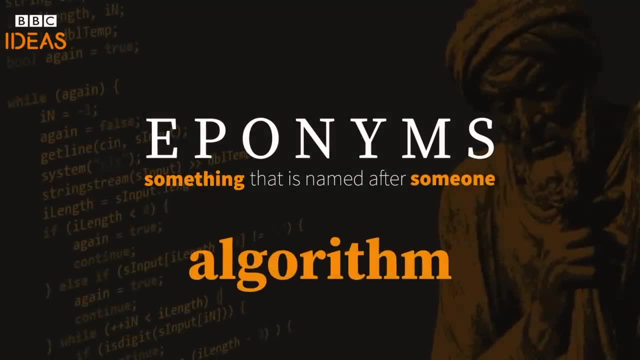 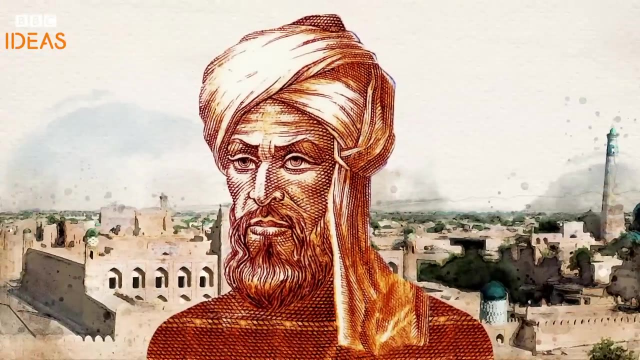 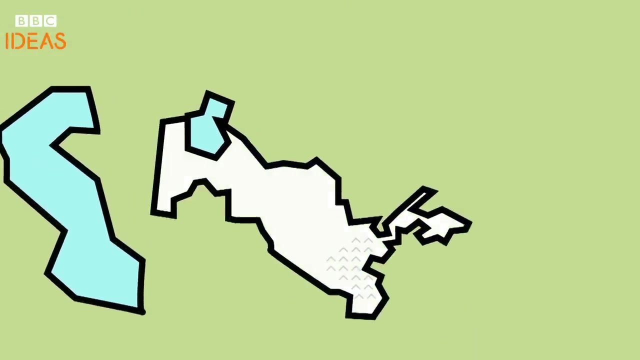 We think of an algorithm as something new, but the term actually dates back about 900 years. The word algorithm comes from the name of a Persian mathematical genius, Muhammad ibn Musa al-Khawarizmi. He was born around 780 AD in the region now known as Uzbekistan. 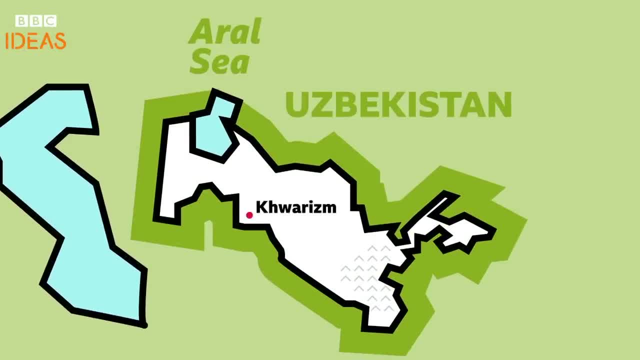 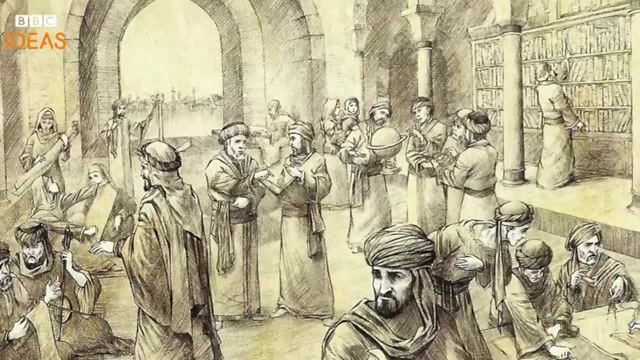 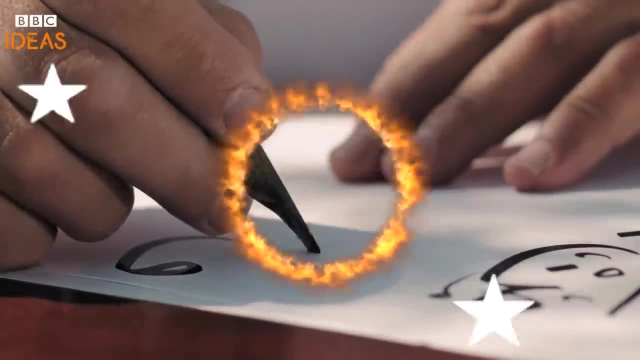 His name suggests he came from Khawarizma. Known as al-Khawarizmi, he was director in the House of Wisdom, an intellectual center for scholars in 9th century Baghdad. He made innovative contributions to mathematics, astronomy, geography and cartography. 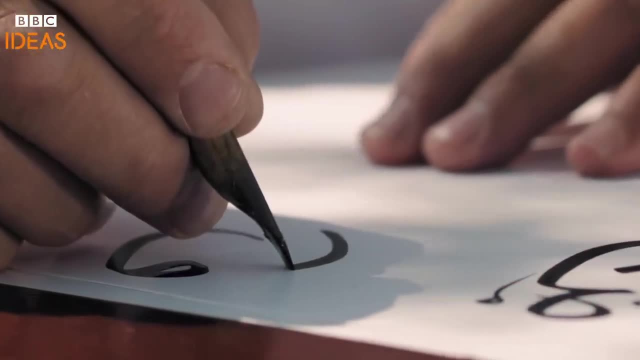 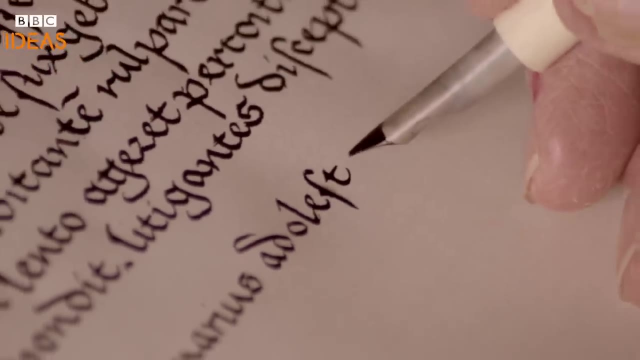 and wrote an influential book called Concerning the Hindu Art of Reckoning. 300 years later, the book was rediscovered and translated into Latin. It introduced Hindu-Arabic numerals to the West, which eventually moved to the Middle East. 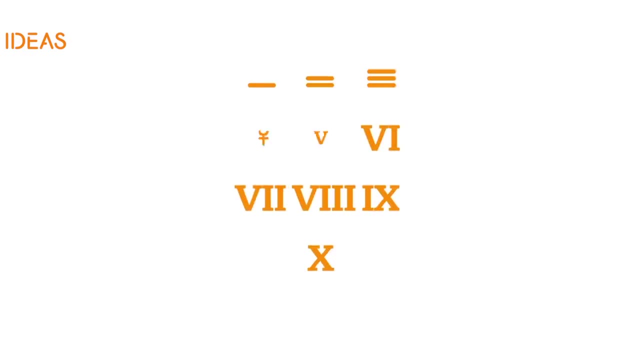 He replaced the unwieldy Roman ones. The Hindu-Arabic number system, along with the decimal point, both described by al-Khawarizmi in his book, are the basis of the numbers we use throughout the world today. Al-Khawarizmi's name, when Latinized in the title of the book, became Algoritmi. 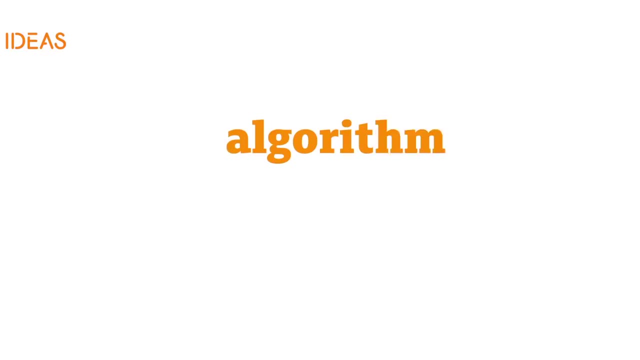 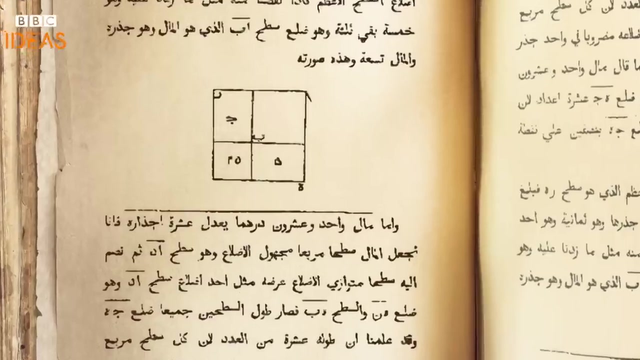 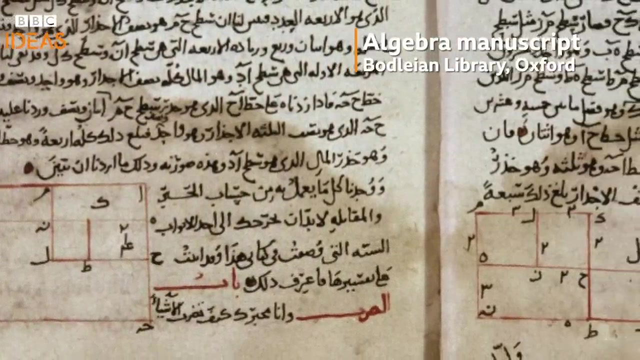 and this is the origin of the word algorithm. We also have al-Khawarizmi to thank for the word algebra, which comes from another of his works. His books revolutionized mathematics in the West, showing how complex problems could be broken down into simpler parts and solved. 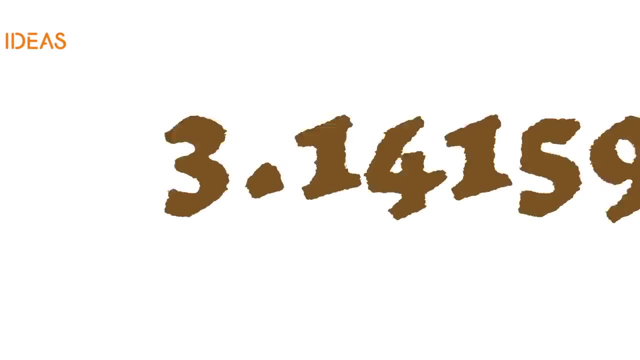 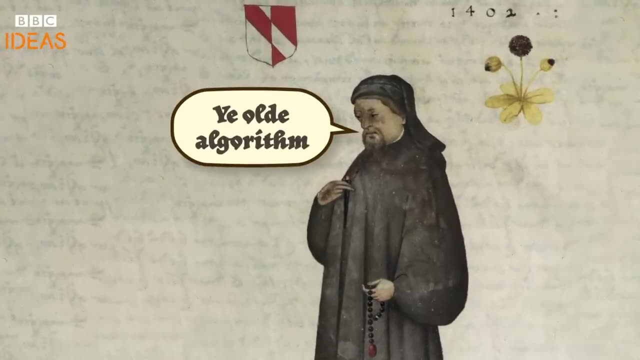 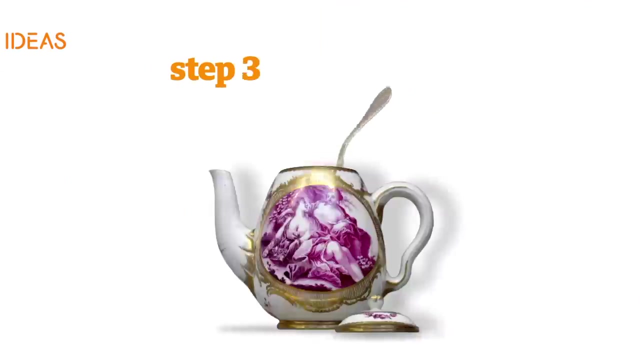 In medieval Latin, Algorismus simply meant the decimal number system. By the 13th century it had become an English word and was used, for example, by Chaucer. But it wasn't until the late 19th century that algorithm came to mean. 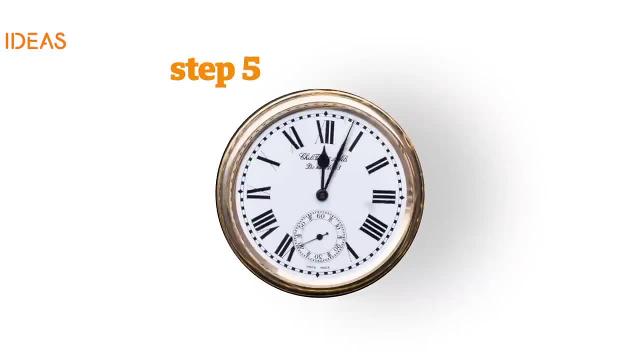 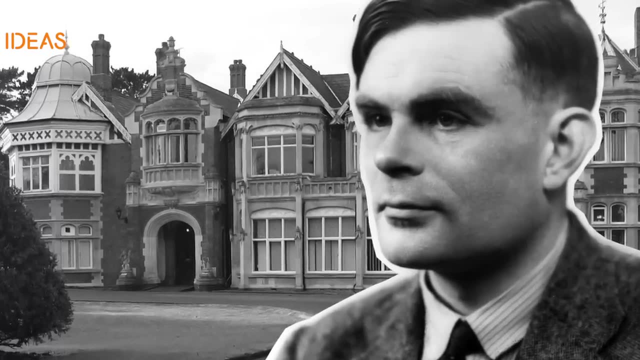 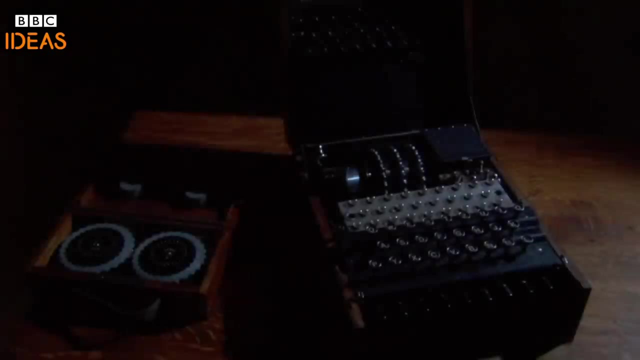 a set of step-by-step rules for solving a problem. In the early part of the 20th century, Alan Turing, the British mathematician and computer scientist, worked out how, in theory, a machine could follow algorithmic instructions and solve complex mathematics.